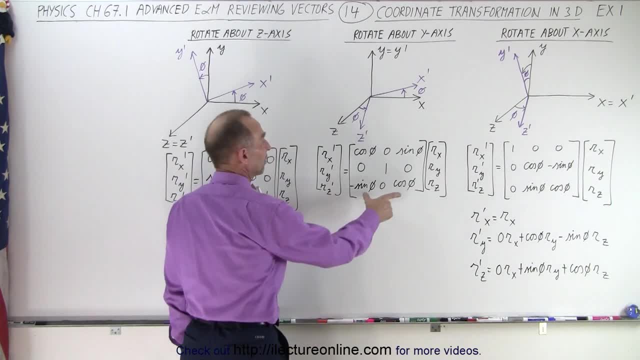 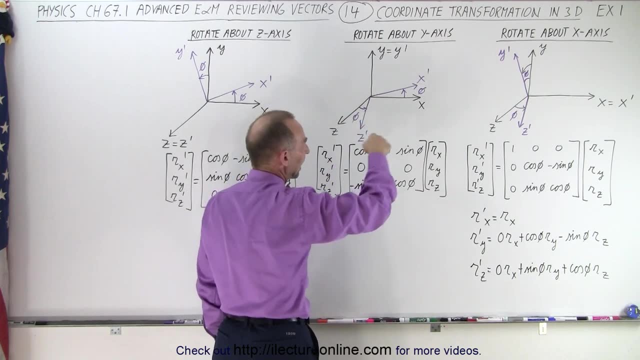 or the same vector in the new coordinate system. So here we have the transformation matrix. When we take the same coordinate system now, we rotate it about the Y axis. So put your thumb straight up and you can see that the X rotates around this way and the Z rotates around this way through an angle of phi. 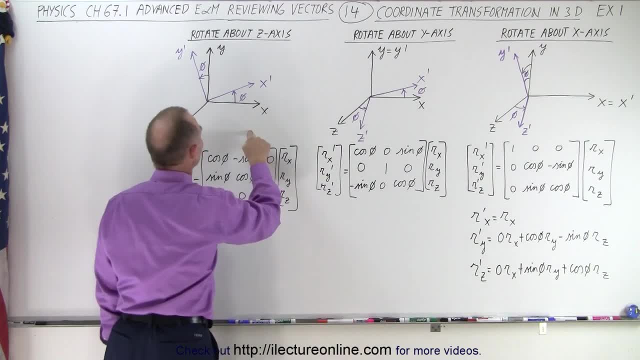 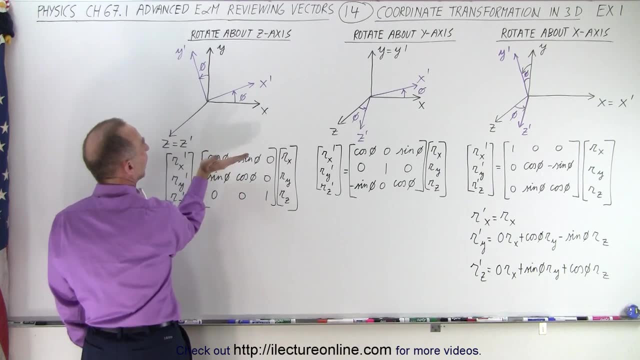 And that's the appropriate coordinate matrix to do that. And then here we take the XYZ coordinate system and now we rotate it about the Z coordinate. So we take the X, Y and Z coordinates. take your thumb point in the z direction and x goes up and y goes to the left, so that the whole 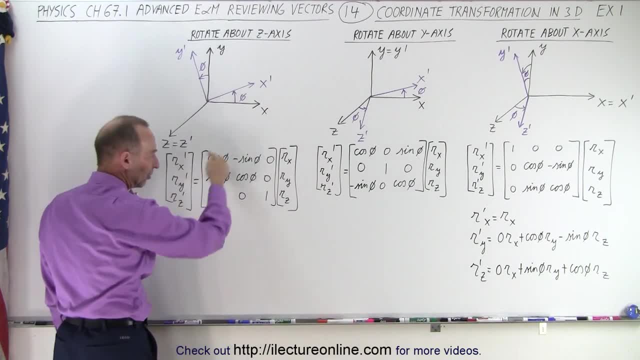 thing rotates about the z-axis to an angle of phi, and this is then the appropriate transformation matrix. Then all we need to know is what is the angle through which we rotate. put the angle values in here and now we have the coordinate matrix or the transformation matrix to go from. 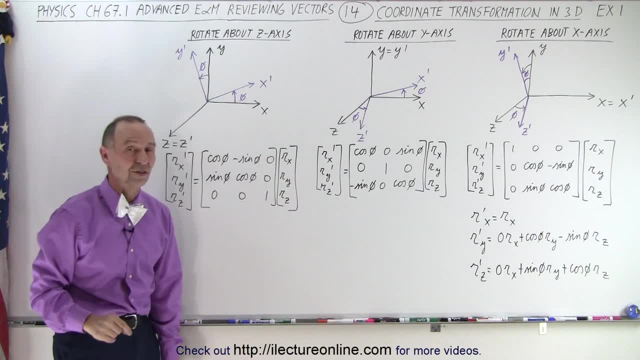 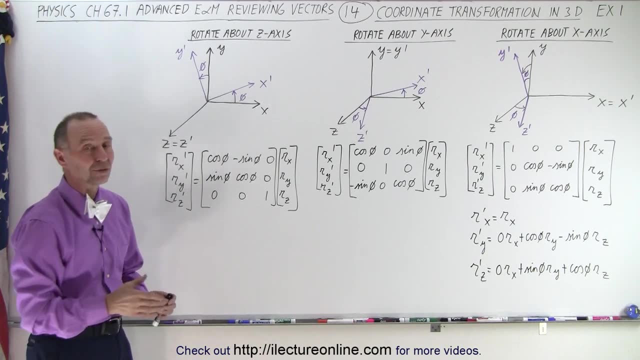 the original coordinate system into the transformed coordinate system, and that is how it's done in three dimensions. Now, to show you how this can be utilized, we'll show you another example in the next video that will transform the coordinate system through a different axis to see how it. 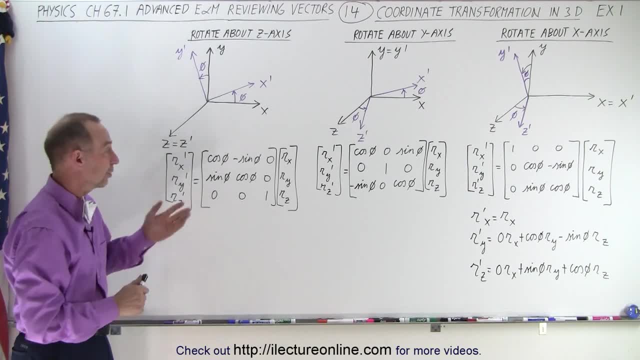 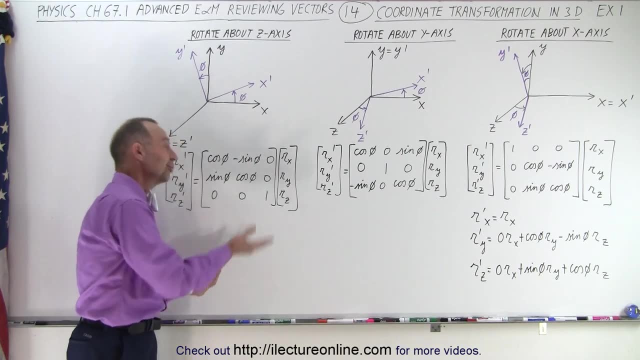 come up with the coordinate system or the transformation coordinate system in that new coordinate system. or let me say that again, it'll show you how to come up with the transformation matrix to then rotate it through the particular axle on the next example. So stay tuned and we'll. 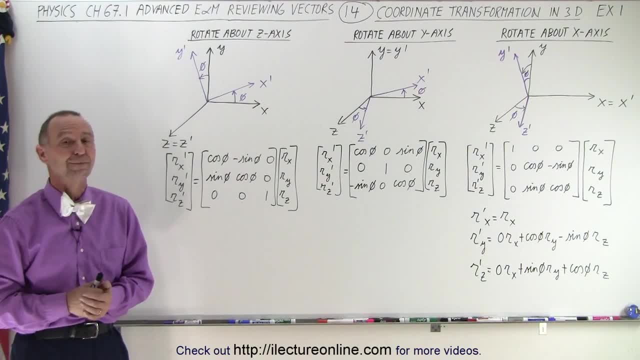 show you one more example in three dimensions so you get more information, More of a feel for it, and that is how it's done.